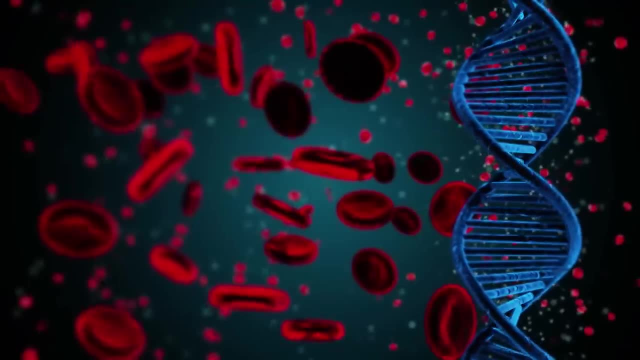 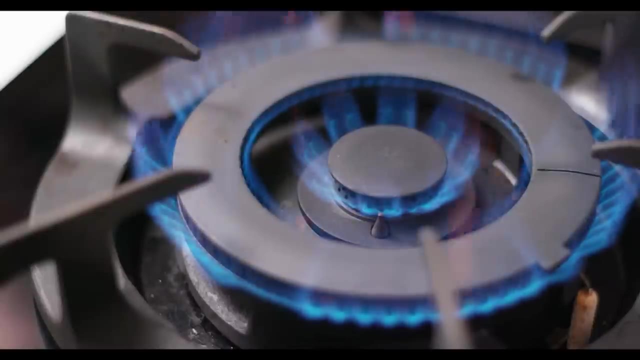 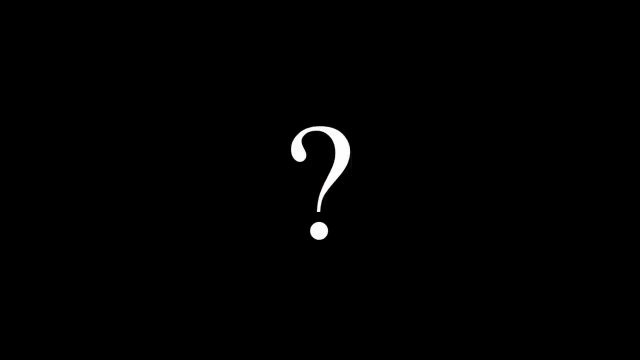 and touch the things made from atoms. Atoms make up the cells that are part of everybody's body and the particles that make up every solid liquid and gas in the world. So if atoms are so small, how do we even know they exist? They're so small you can't even 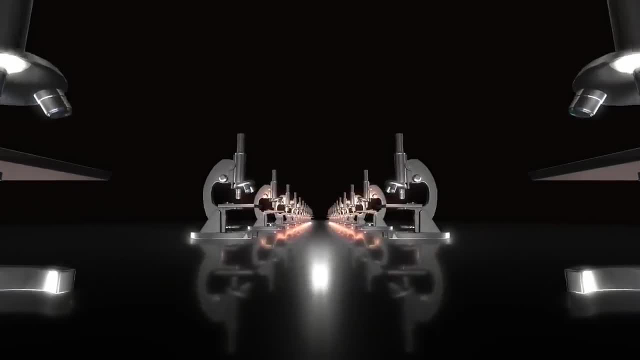 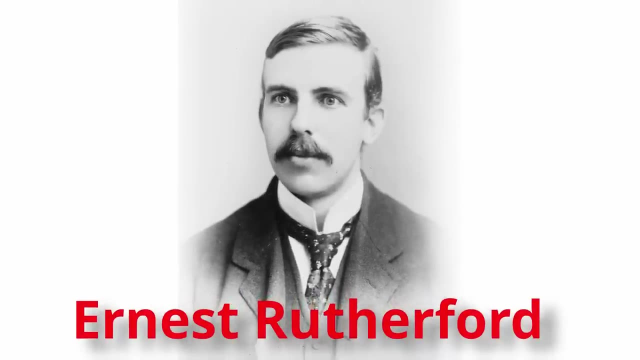 see them with the highest powered microscopes, But we do know they're there. That's because more than a hundred years ago a scientist named Ernest Rutherford was able to bounce other small particles off of atoms and witness the interaction. It was kind of like you. 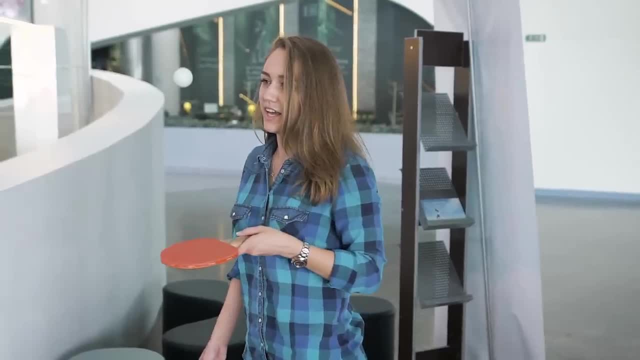 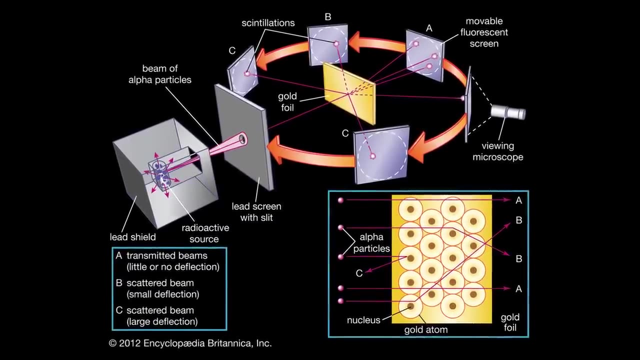 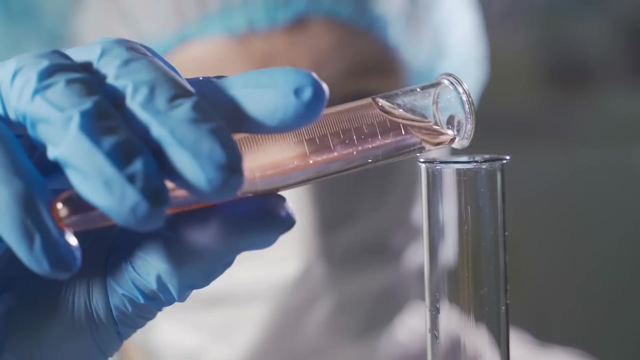 bounced a soccer ball off a tiny, tiny super ball. The way that super ball- or, in Rutherford's case, atoms, acted told him they existed and what they were made of. This history of how atoms were discovered is a lesson for another time, But scientists have proven the existence of atoms. 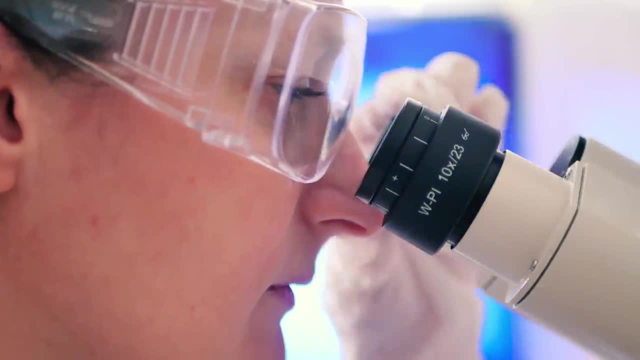 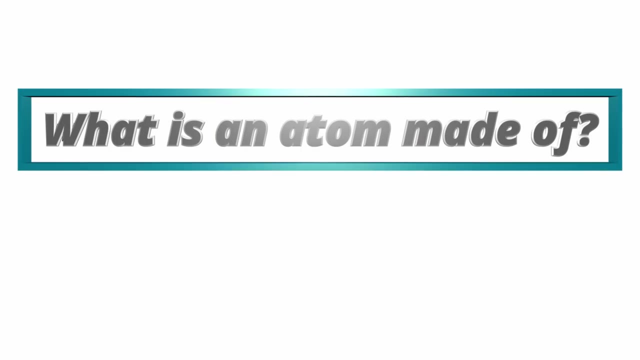 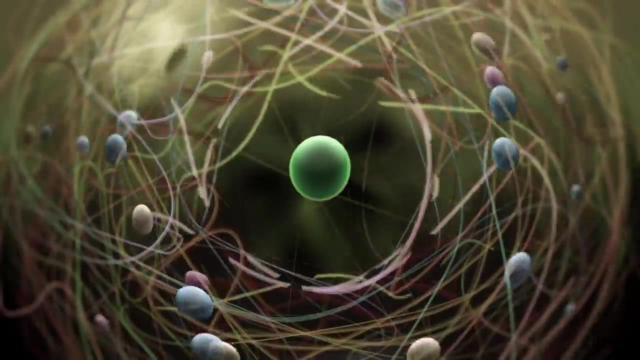 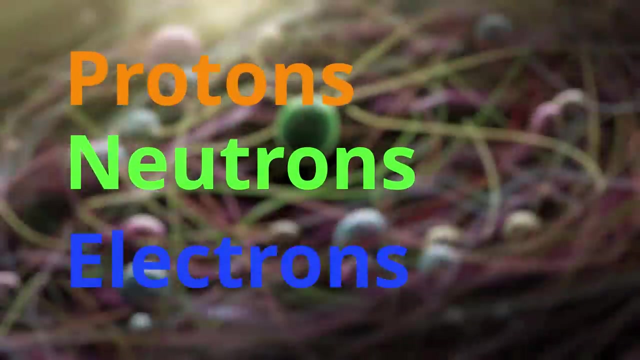 in many different ways over the last century. They're definitely there and they're really cool. So what is an atomator And how does it behave? It's hard to believe that inside every atom there are three even smaller particles. These particles are known as protons, neutrons and electrons. The difference? 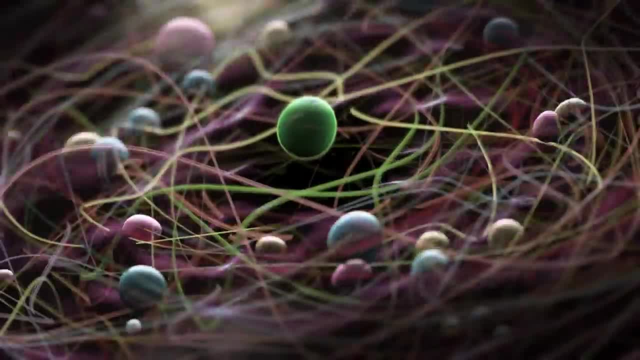 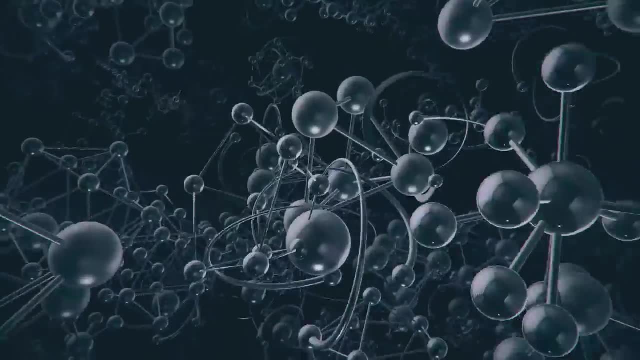 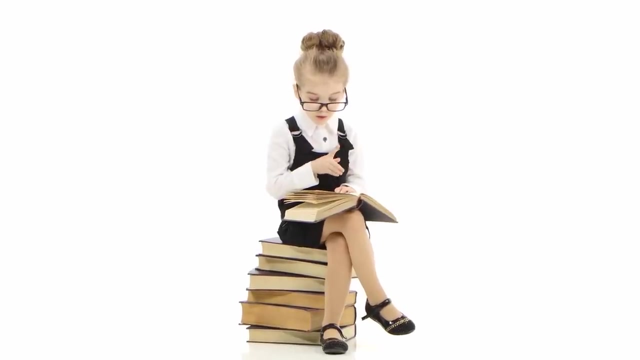 in the way these three particles exist within every atom and the way they interact with other atoms help determine what these atoms create. These atoms make up wood or water or water Or metal or anything, But we'll get to that shortly. 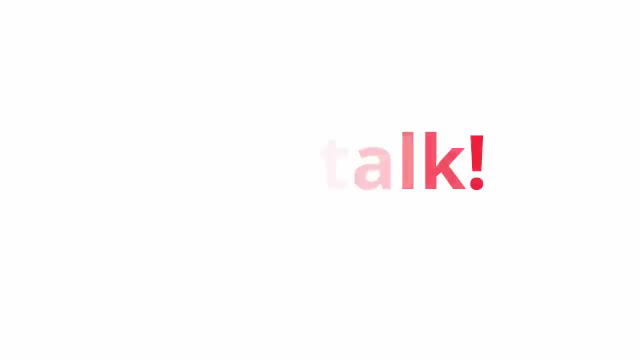 First let's talk about these three particles: Protons, neutrons and electrons. A proton carries one unit of positive electric charge, An electron carries one unit of negative charge And a neutron has no electric charge. Together, the protons and neutrons make up the nucleus. 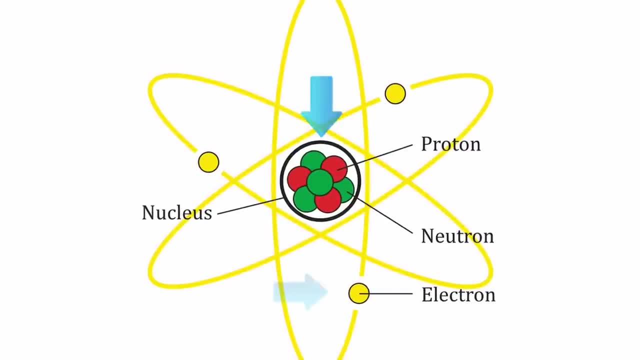 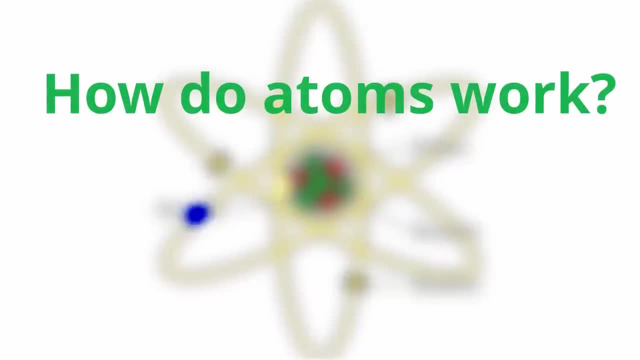 of an atom or its nucleus. So what is an atomator? Well, an atomator is a particle. It has two electrons, one at the center and the electrons spin around the outside of the nucleus in what is called a shell. How do these super tiny atoms work And what do? 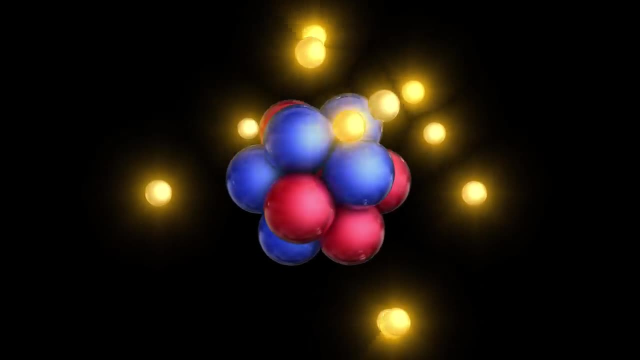 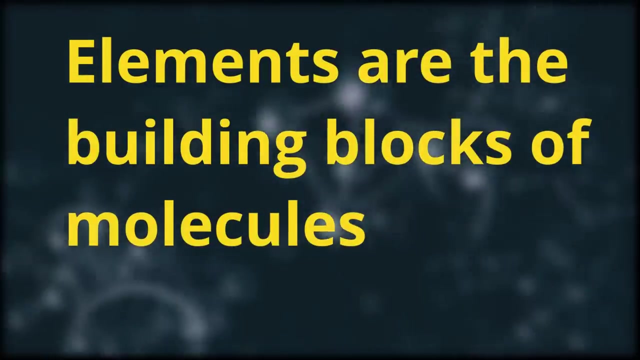 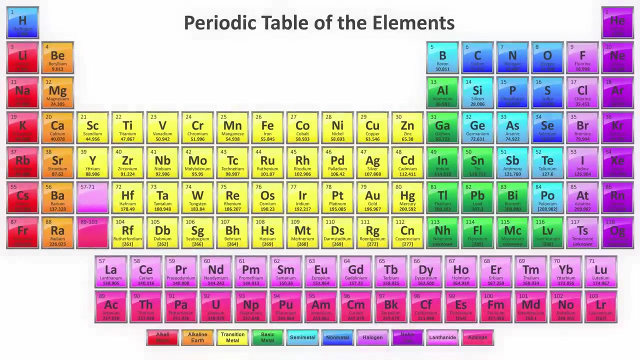 they do. The different ways that atoms are organized determines what they are or what elements they make up. Elements are the building blocks of molecules, and everything around us consists of molecules. All the elements are different, and there are a hundred and twenty of them. 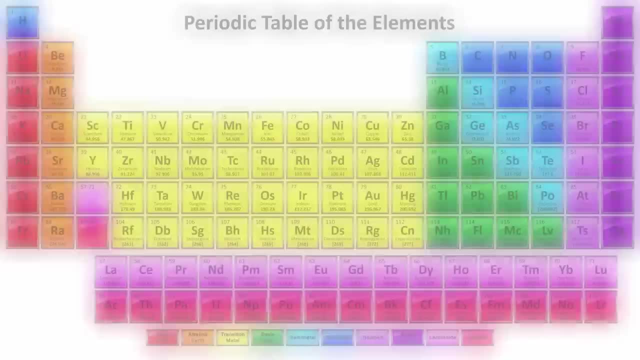 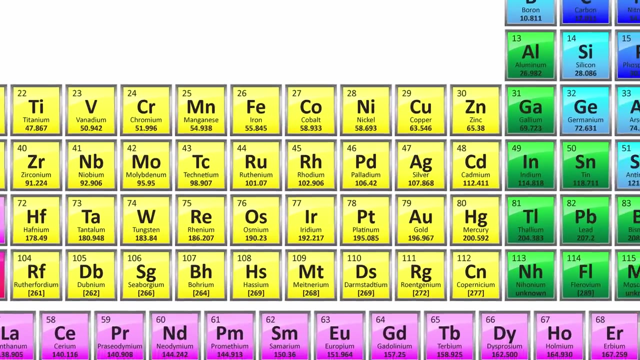 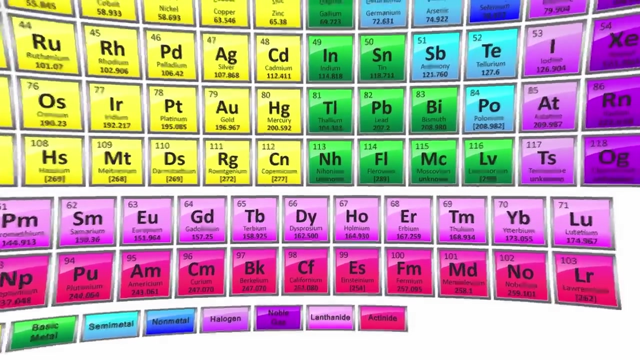 These 120 elements are laid out here in the periodic table of elements. This chart is used by scientists like physicists and chemists to study how solids, gases and liquids behave. It all depends on what they're made of. You'll probably spend a lot of time studying this chart later, as you continue learning about. 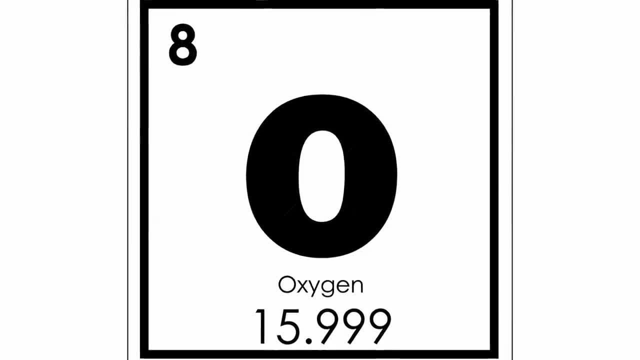 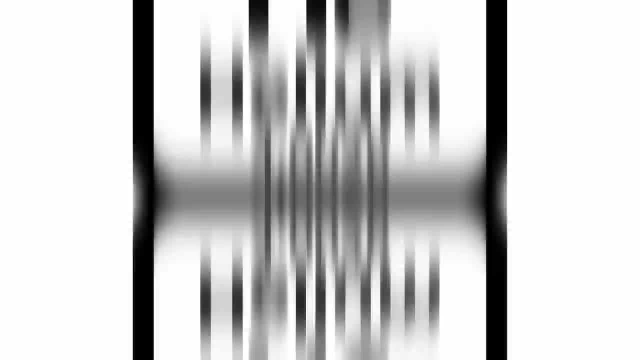 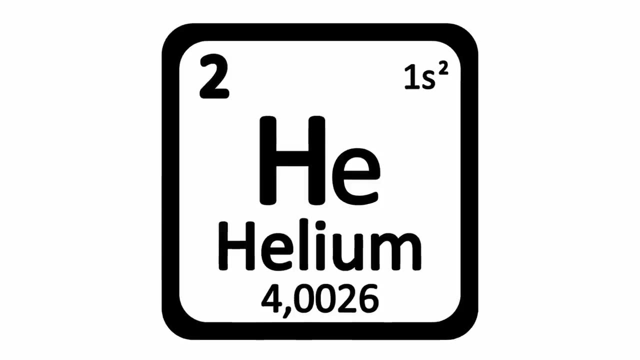 science. This is the element oxygen. The number 8 means that the atoms that make up oxygen have 8 protons. This is helium, and its atoms have 2 protons. The number at the bottom tells us what the atomic weight of the element is. As you can see, there are 120 such elements. 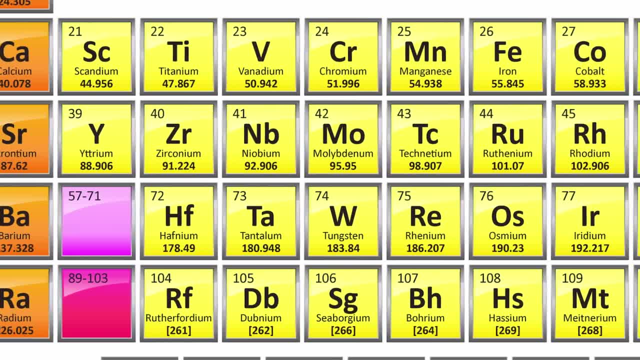 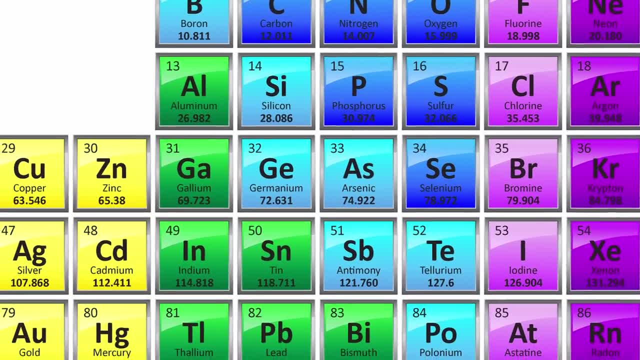 on the periodic table, and each of those elements is made up of atoms. Think of it this way, Just as the letters in the word tell you what the word is: the number of protons, neutrons and electrons that make up the atoms in an element. 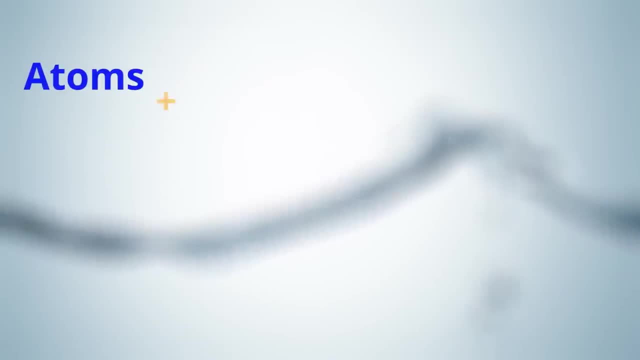 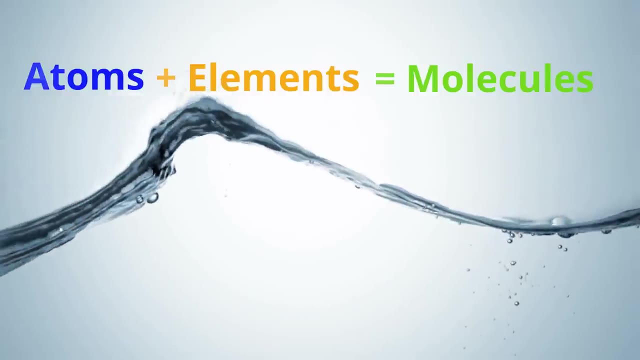 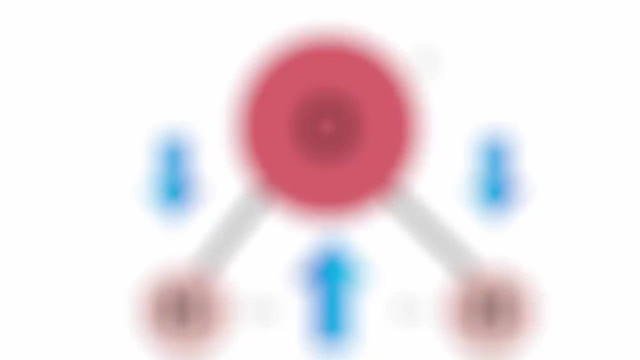 tell you what the element is, And when atoms and elements are joined together, they make up molecules. Water, for example, is a molecule. Each water molecule is made up of two hydrogen atoms and one oxygen atom, and is sometimes referred to as H2O2.. Water, for example, is a molecule. Each water molecule is made up of two hydrogen atoms and one oxygen atom and is sometimes referred to as H2O2.. Each water molecule is made up of two hydrogen atoms and one oxygen atom and is sometimes referred to as H2O2.. 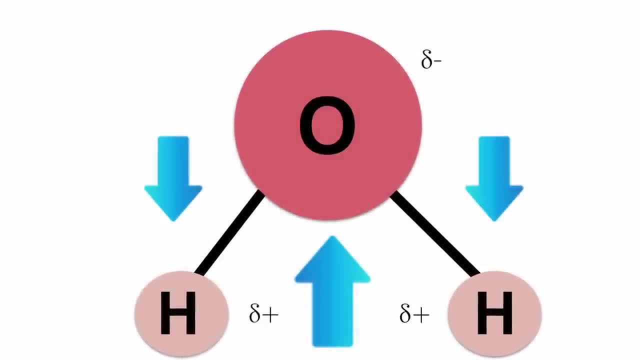 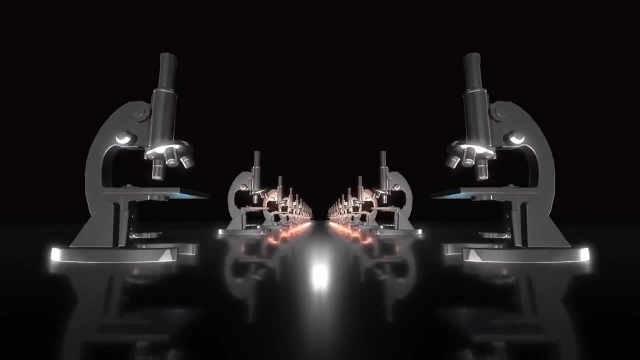 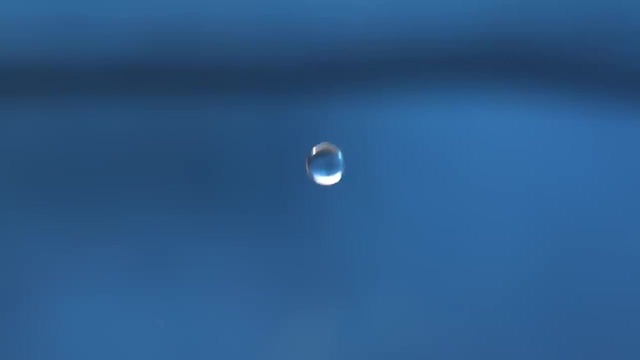 It takes two atoms of one hydrogen and one atom of oxygen, to make water. As we said, atoms are super tiny and therefore the molecules they create are also really, really small and can't be seen without a special microscope. Think about it. Can you see a single molecule of water? No way, Even the smallest drop of water.